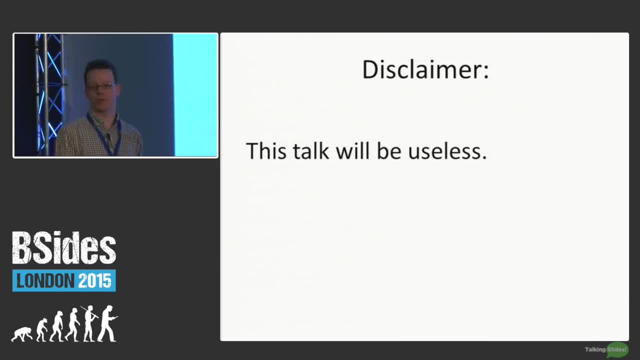 mathematics, which you can't squeeze into a year. You definitely can't squeeze it into a 45-minute lecture. If you were expecting to learn anything useful, you probably should go To one of the other rooms. I also don't want to stand here pretending I'm a cryptographer. 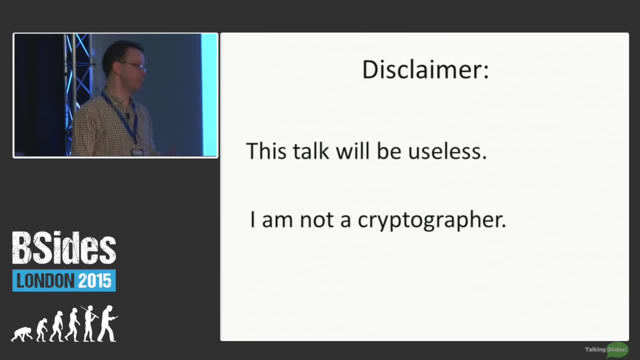 I understand the math because I used to do that. I could implement the algorithms, but I'm a sloppy programmer. I would probably make a few mistakes. I wouldn't be able to find fault in other people's mistakes and I don't know all the details of the research. 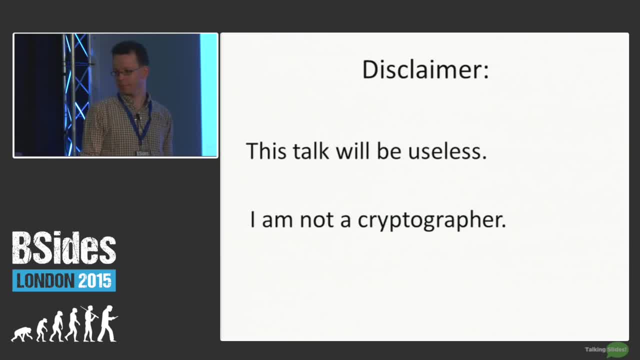 what to look for in implementations. And finally, I'm really. This talk is really aimed at people who don't have much understanding of mathematics, so I skip over some of the gory details. If you happen to know a bit about elliptic curves, 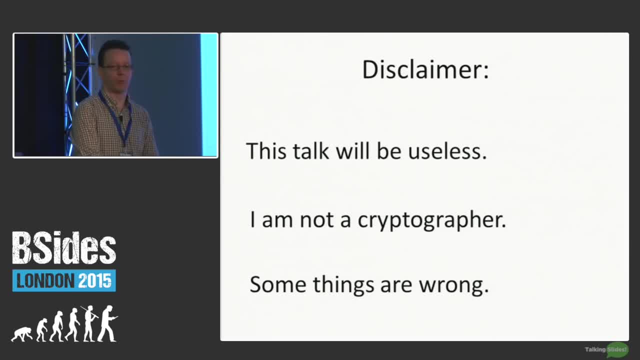 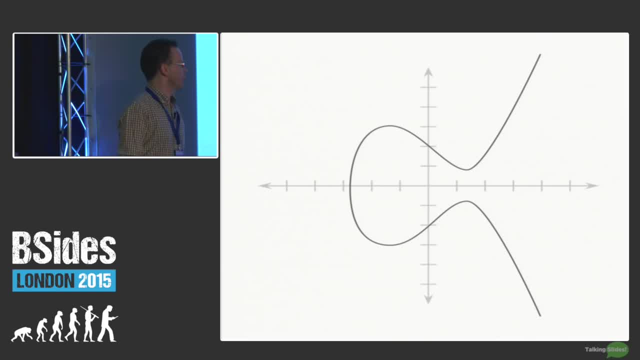 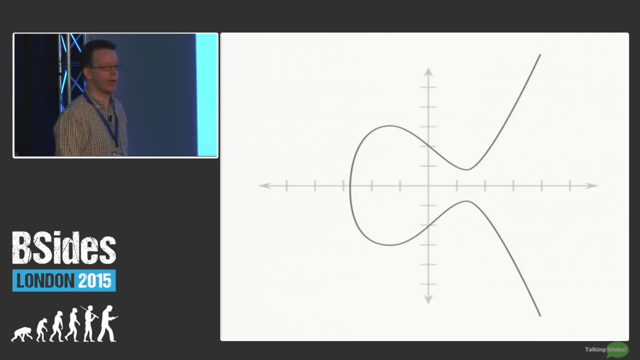 this and you see the curve. you see the X and the Y axis in the background, And on this curve there are a very large number of points, And it is these points that play a role. Now. computers can easily represent these points by their coordinates or just. 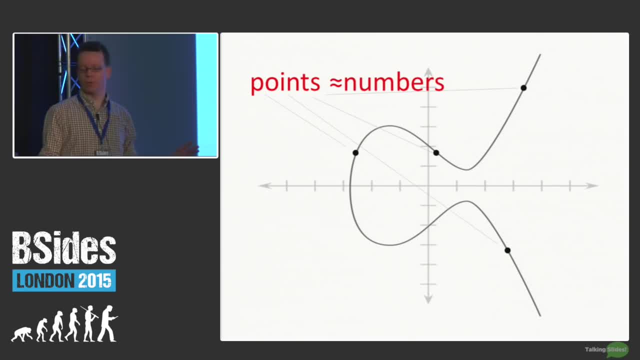 by numbers And in this talk I will assume that points are numbers And from a computer's perspective, standards are always very scared of scoring size. This is more or less true. It's one of these details matter a lot because that's where you could make mistakes. 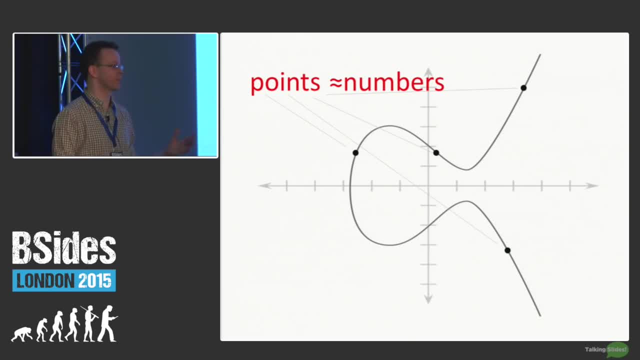 but I'll just assume that a point is represented by and represents a number. The most important property or one of the most important properties of elliptic curves is, if you take two points on the curve, P and Q, and you take the line through P and Q. 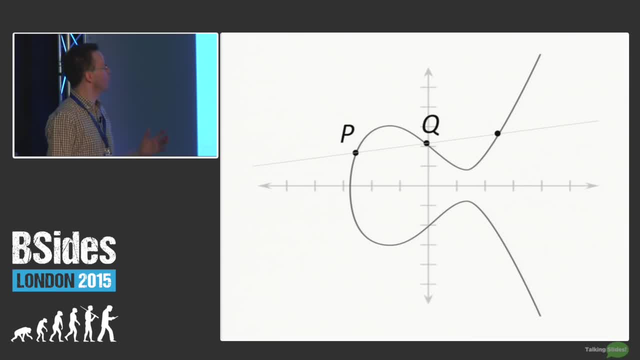 there's always one line. there's one such line. then there is a unique third point on the curve on this line, And a second important property is that the curve is, as you can see, symmetric in the horizontal axis, the X axis. 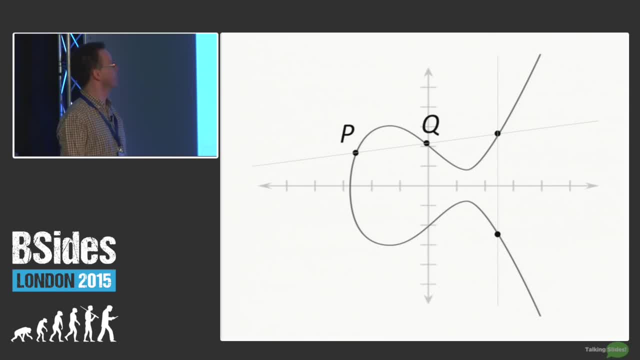 You can take the vertical line through this and you get another point on the curve. At this point we call P plus Q. I can't emphasize enough that this is not supposed to make any sense. This is just a definition of you define P plus Q this way. 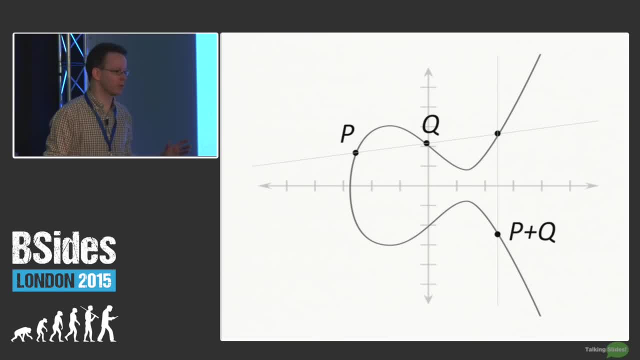 If you're studying mathematics and you learn about elliptic curves for the first time- which would make you a minority because within mathematics it is a bit of a niche subject- if you would learn this, it wouldn't make sense either. There is a bigger theory behind this. 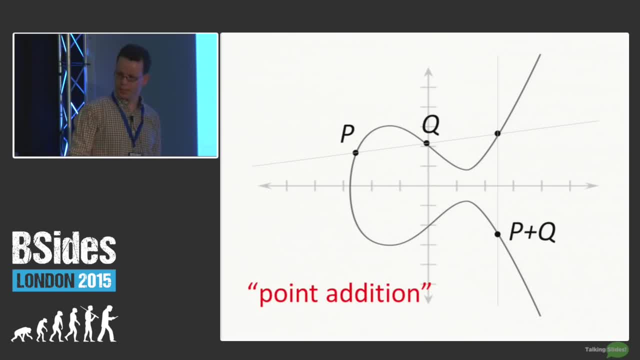 but this is like even more advanced math And this is what we call point addition on an elliptic curve, which means, for every two points on the curve, for every two P and Q, wherever they are, we can define the third point. 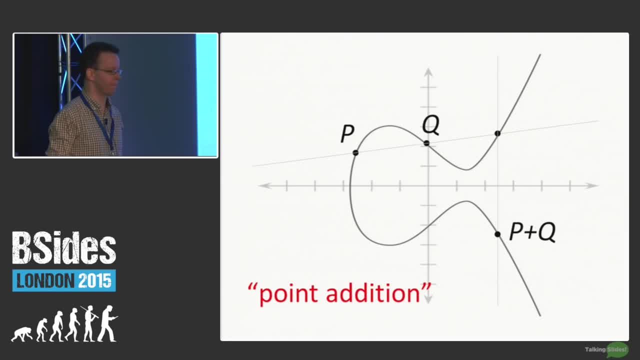 which we call P plus Q. That's another point. That's another point on the curve. And the second nice property is if you take a point P on the curve, well, you may wonder, some of you may wonder what, if you want to define a point P plus P. 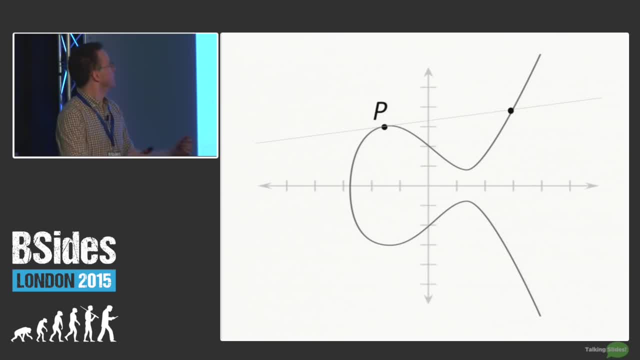 Well, you take, there's a unique line through P that touches the curve. It doesn't go through it. It's called a tangent line to the curve at P. This line has a. it's also a unique extra point that goes through the curve. 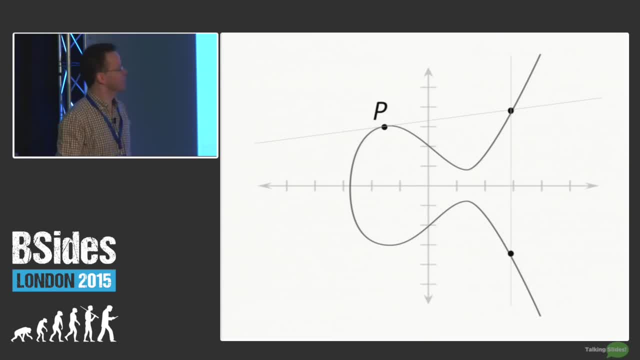 that lies on the curve and on the line, And again you can take the vertical line through it and you find a point P plus P And we actually call this two times P And this is called point doubling. You can double a point. 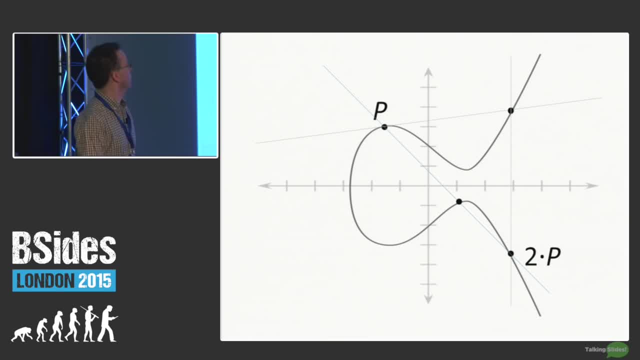 And you can combine it. You can get two P plus P. Again, take the line through it, take the vertical line, and you get a point: two P plus P And, as you may have guessed, this is called three times P. 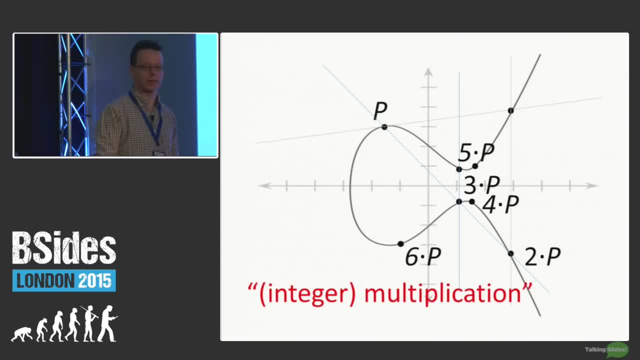 And you can get four times P and five times P and six times P, et cetera. This is called multiplication or integer multiplication. You take a point and a number and you take the number N, you take N times that point, for whatever N is. 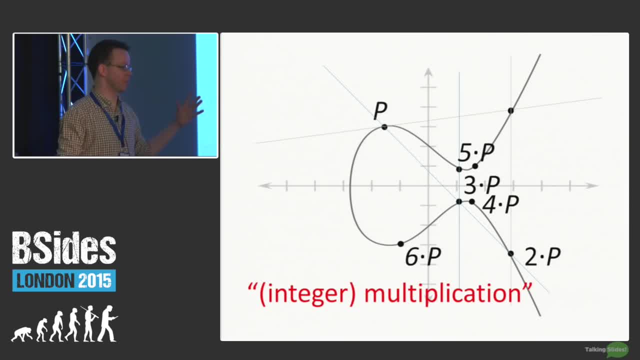 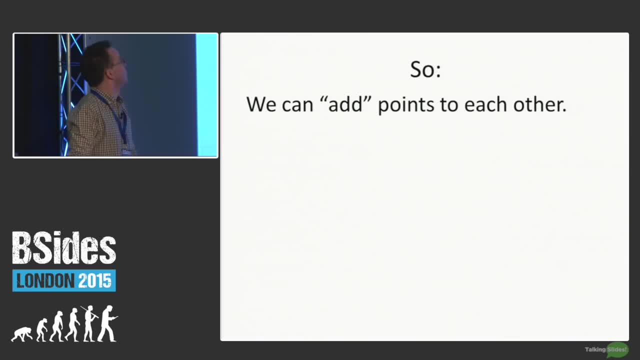 And this is the algorithm. computers can implement it And computers are very good at that. So so, yeah, So, so, so we can add points to each other. Take for points P and Q. we define, we define a point P plus Q. 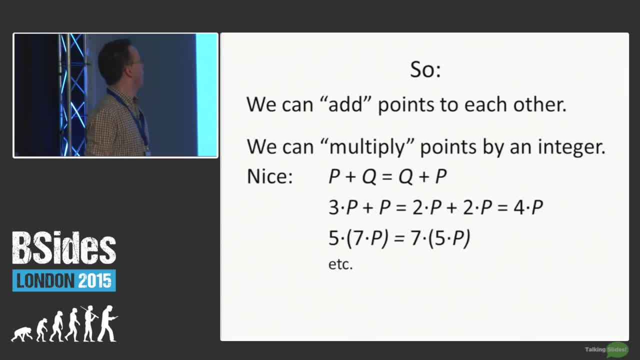 We can multiply points by an integer And it happens, and you don't have to worry about this. but this all satisfies nice properties. If you add P, P plus Q is Q plus P, et cetera. This, this means that the points form in a billion group. 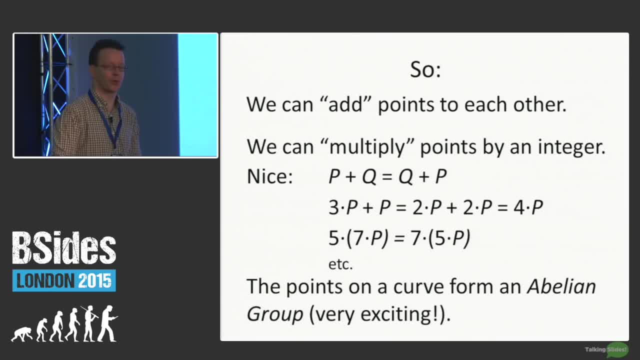 You don't have to know what it means, You don't even have to remember this, but if you're a mathematician or a cryptographer, this is extremely exciting, And mathematicians don't get excited very much. Now it happens that multiplication by integers is very fast. 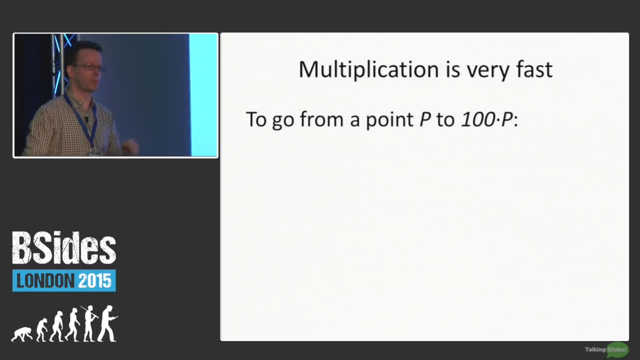 So if you had a point P and you want to get the point a hundred times P, then the algorithm I just showed, which you can implement in a computer, uh, you just add P 99 times to this point P, You get P, two P, three P, four, P, until you get. 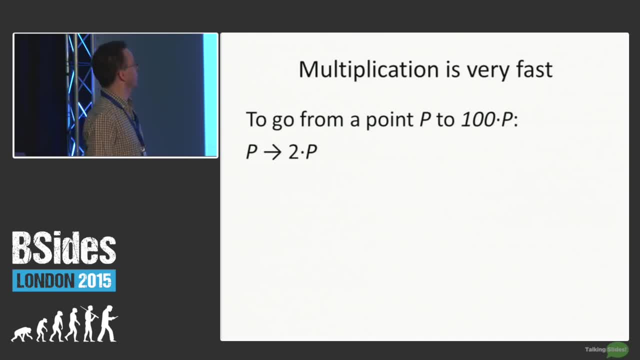 a hundred times P. However, computers can do this much faster And as follows: you take P, you double it, you get two times P. Next step is: you add P to it Three times P, double it again six times P. 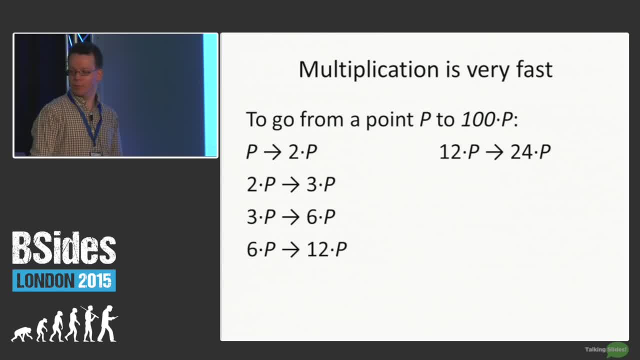 double it again 12 times P, double it again 24 times P, then you add P to it. you get 25 P times P. then you double it again 50 times P and double it again a hundred times P. 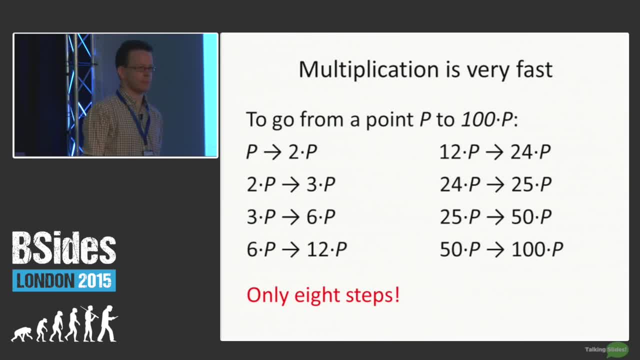 So these are eight steps rather than 99.. If, if you start to multiply by integers of 50 digits or more- and this is what happens if you do elliptic curve, cryptography the this is extremely fast. I mean eight or 99, for a computer doesn't make a difference. 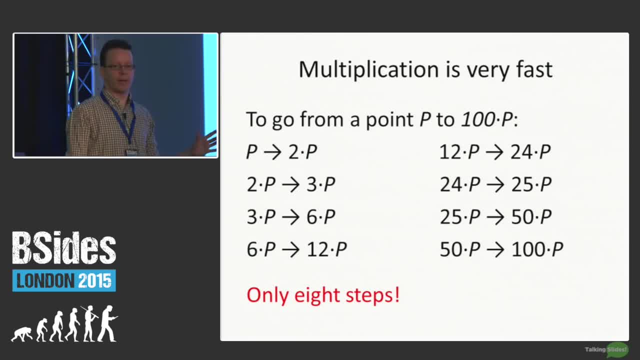 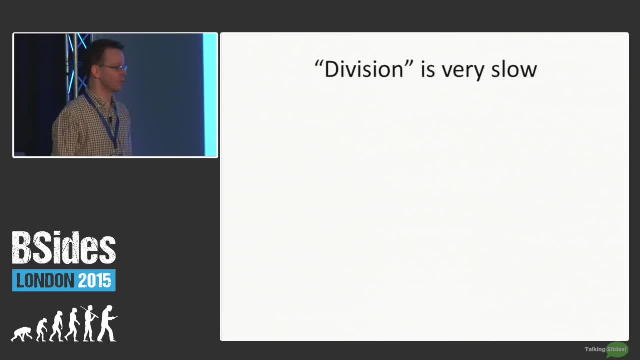 but we're really talking about many, many orders of magnitude. However, the other way around, which I call, but isn't officially called, division- uh, it's very slow. So imagine you have two points on the curve: P and Q. 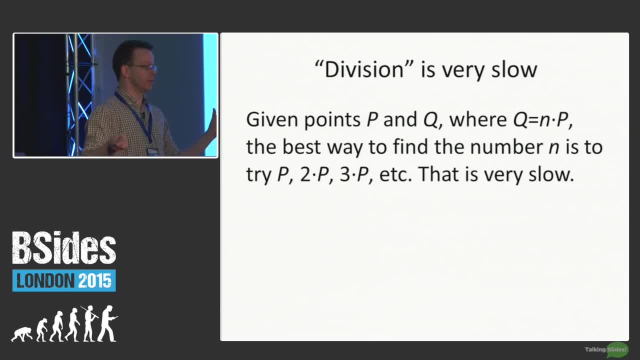 and you know that Q is N times P for some number, N It could be a hundred, it could be a million, it could be 17, quintillion. You don't know really the best way, almost the best way, to find this number. 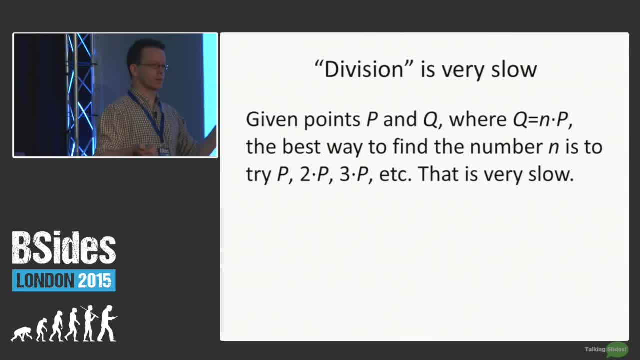 N is to start with P, then get two times P, three times P, four times P, until you read, you reach the point that's Q, and then you know the number N. This is an extremely slow process And, as I mentioned, 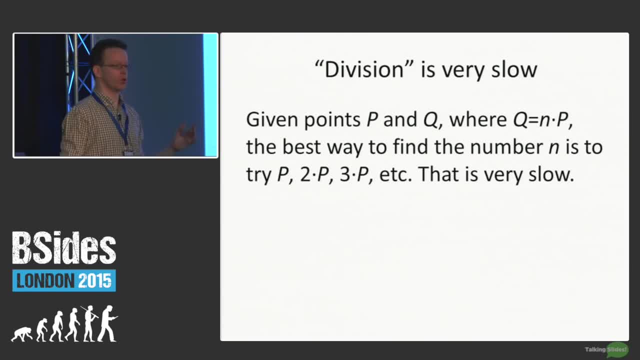 if N has, if N has 50 digits, um, this is just undoable for a computer, even for a fast computer, even for the kind of computers that I have in a data center in Utah, And this is called the discrete logarithm problem for elliptic curves. 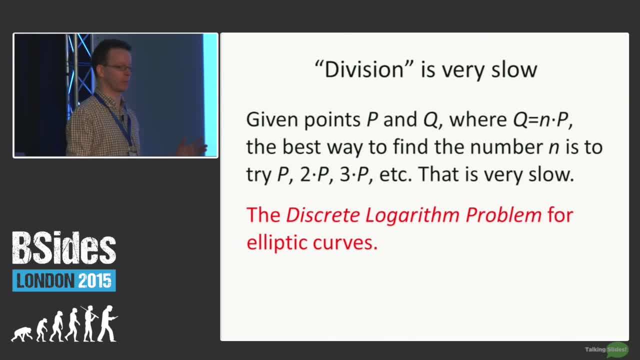 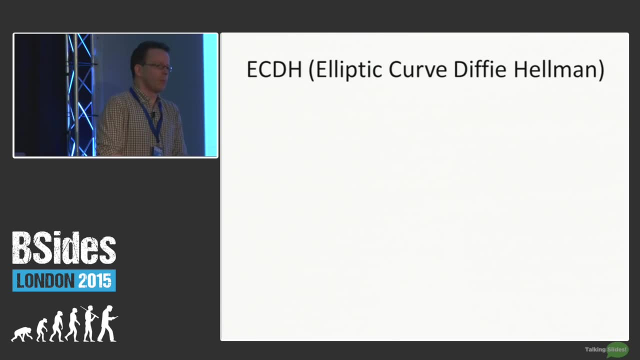 And it's this that is the basic basis of elliptic curve cryptography: The fact that multiplication is fast but division- or taking a logarithm is officially called- is very slow. So the most important, or probably the most important uh kind of elliptic curve cryptography is to elliptic curve. 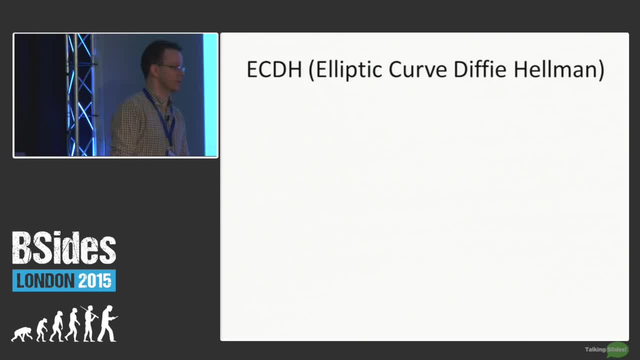 Diffie-Hellman algorithm, ECDH and sometimes elliptic ECDH-E. What is for a femoral? but that's irrelevant for now. It's used in the following way: or or to get to solve the following problem: two entities. 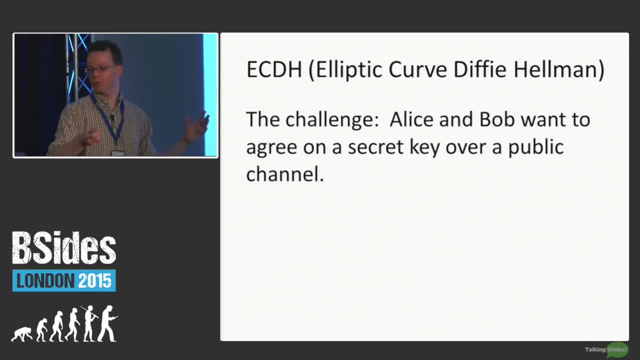 let's call them Alice and Bob, because we're doing cryptode. They want to agree on a secret key over public channel, For example. For example, Alice is a web server, Bob is a web browser and they want to agree on a secret key. 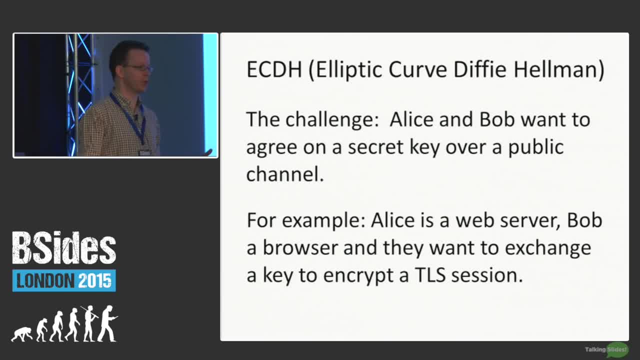 so that they can encrypt their connection. There are very fast algorithms like AES where, as long as you have agreed on a secret key, then you can encrypt the whole connection very quickly, very fast, in real time. However, how do you agree? 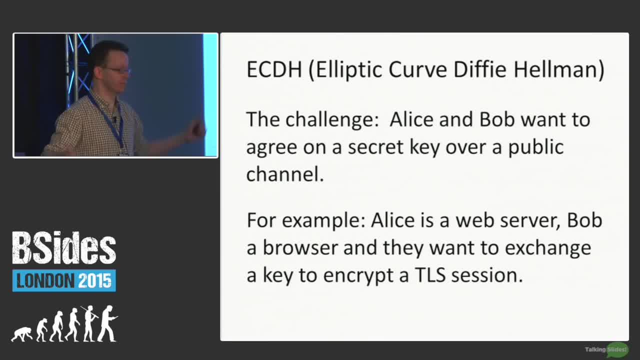 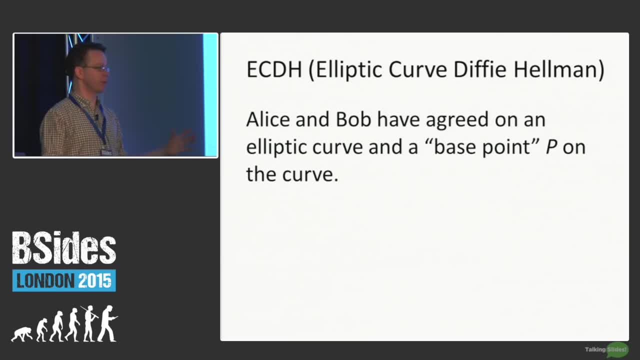 Because before you start encrypting, nothing is encrypted and anyone can read anything. So the algorithm is as follows: First, they agree on elliptic curve to use- and, as I said, there are many different curves- and the base point P on this curve. 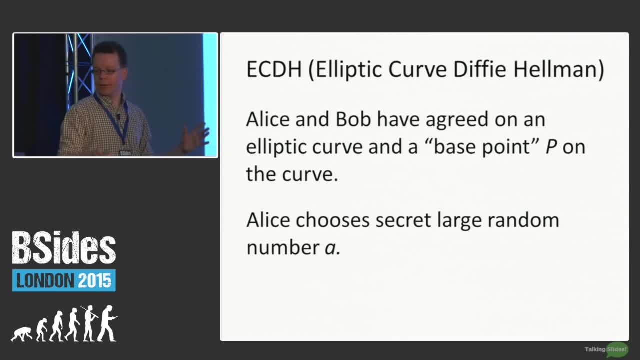 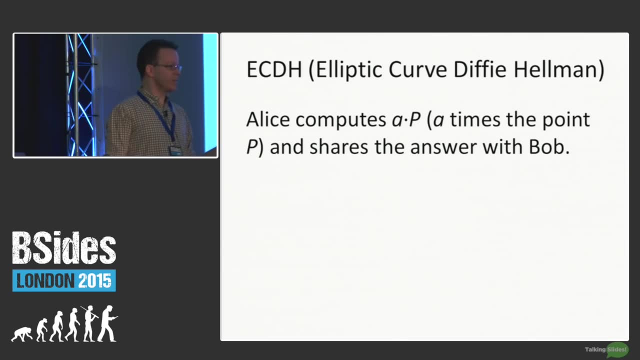 Alice then chooses a large random number A. She doesn't tell anyone about that, She just keeps it to herself. And Bob chooses a large random number B, lowercase b. Now Alice computes A times P, And even if A is very large, 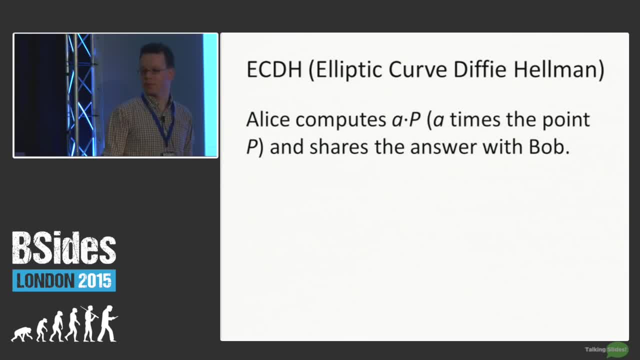 we've seen, or I've shown, or at least I've told you that this is something her computer can do very fast And she shares this number, or sorry, this point, which is kind of a number A times P with Bob. 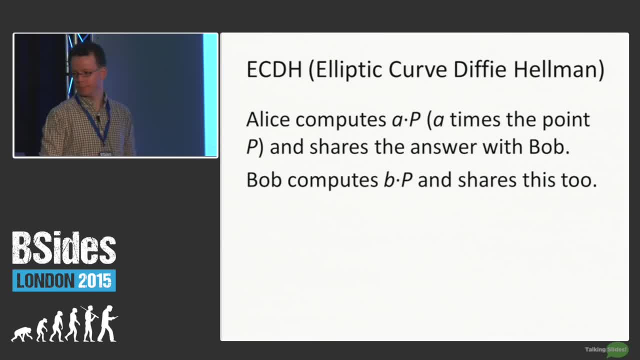 over a public channel. She doesn't care if anyone can read it. Bob does the same with his secret number. He computes B times P B. he keeps secret, but he shares the resulting point slash number B times P with Alice over a public channel. 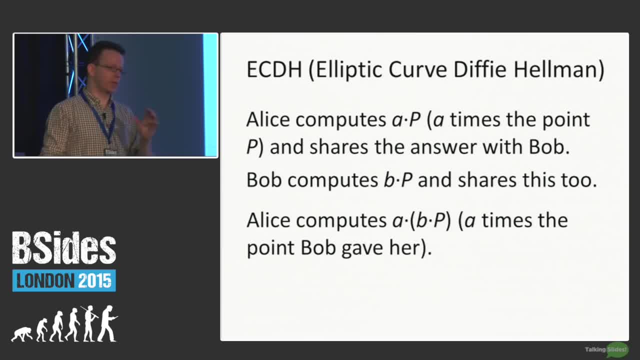 Anyone can read it. Now. Alice has been given B times P. She has the secret number A and she computes another point: A times this point, B times P, which is another point on the curve. Bob computes A times P, so B times the point. 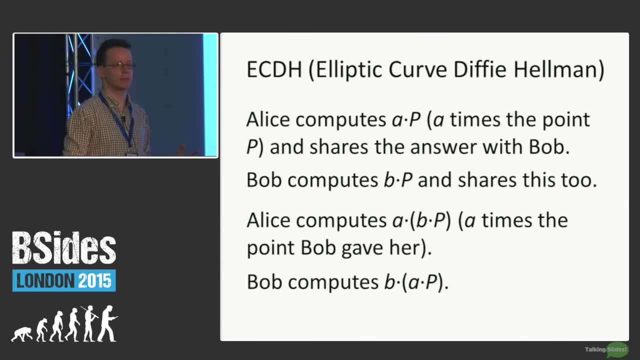 that Alice has given him over the public channel using his secret number B And they get a secret key because A times B times P is B times A times P. So they have agreed on a shared secret number and the discrete logarithm problem. 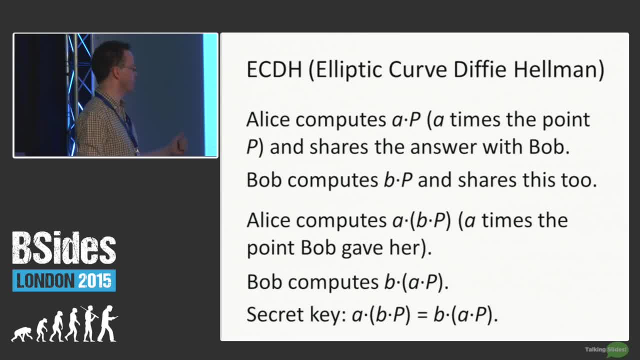 means that no one can correct this. even if they can read, even if they know what curve is used, if they know the point B, if they have seen A times P and have seen B times P, You can actually see this in wires. 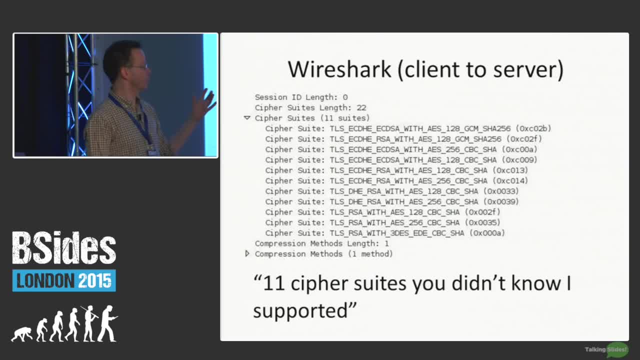 and this is a wireshark session from Firefox on Debian Linux connecting to the website of Bsite London over HTTPS, And wireshark actually shows it. The browser tells the server. well, I know a number of cipher suits. Cipher suits is a series of algorithms. 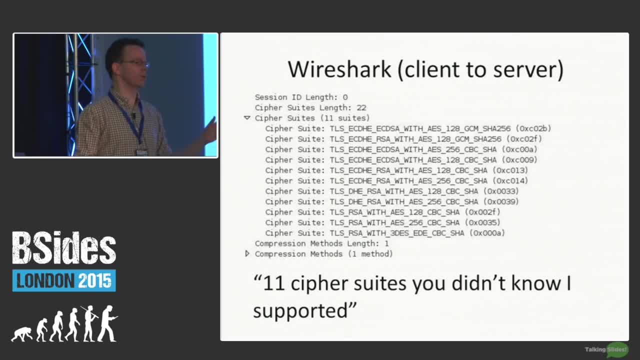 because in TLS or in HTTPS you need multiple encryption algorithms for different things, And the first six that are listed they say ECDH or ECDHE, which is the algorithm I just explained. So the client, the browser, tells the server. 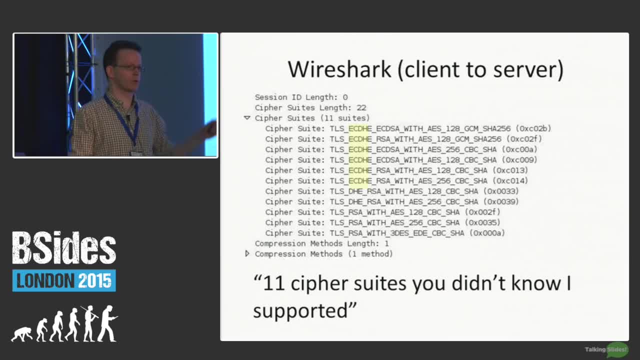 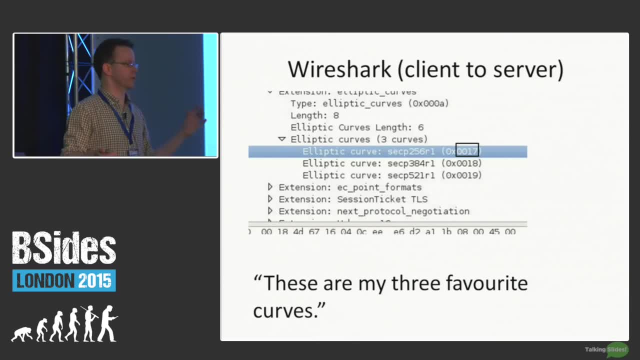 well, I support these 11 algorithms, in this order of preference. And the client also says these three curves. these are publicly known curves defined in standards. these are the curves that I support. So if we're going to do this, we're. 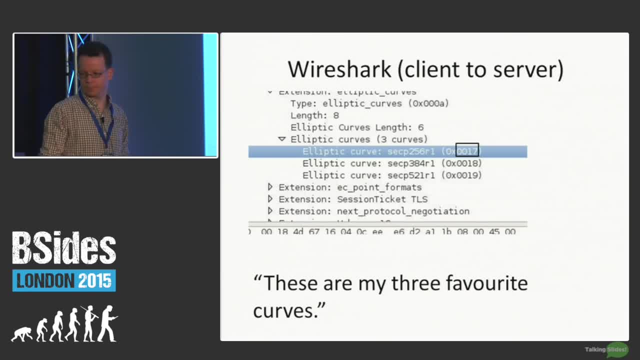 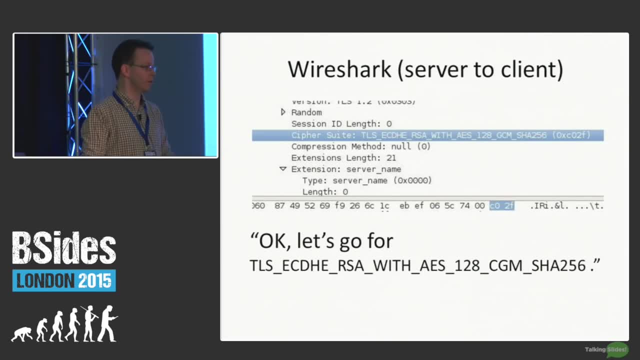 going to do elliptic curve, Diffie-Hellman, use one of these three curves And the browser responds: sorry, the web server responds and they say: OK, one of these algorithms. indeed, using elliptic curve, Diffie-Hellman. 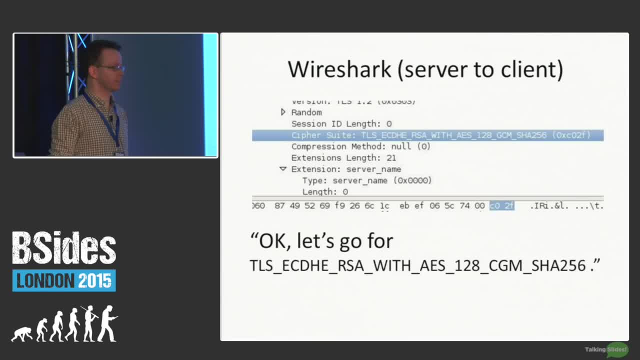 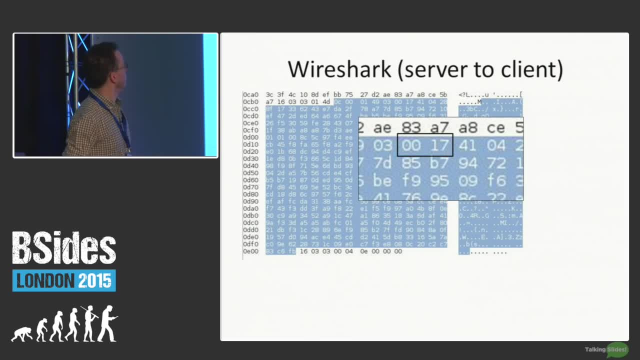 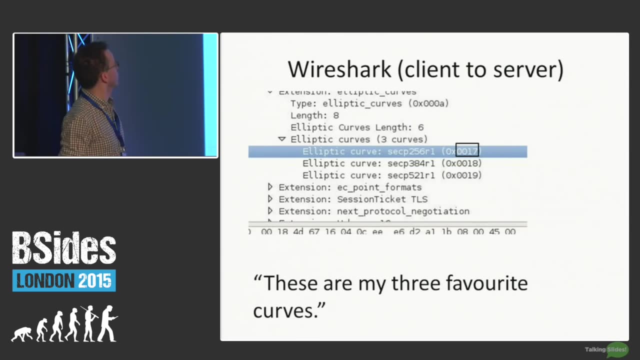 and a number of other things. Let's go and use that. And then the server also says: yeah. the server- sorry, I should have pointed out here. when the browser tells the server three curves that it supports, they have numbers. 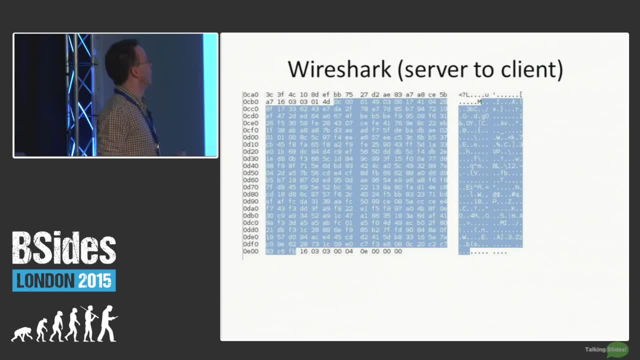 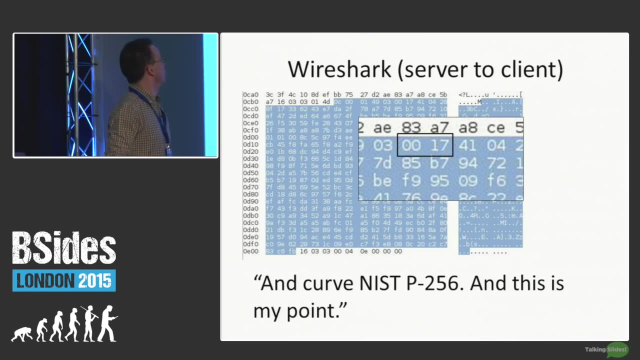 And one of them is hex 0017. And the server tells the client: OK, 0017, that's the curve we're going to use. That corresponds to NIST P256, which is a curve, And most of the other blue stuff, what you see here. 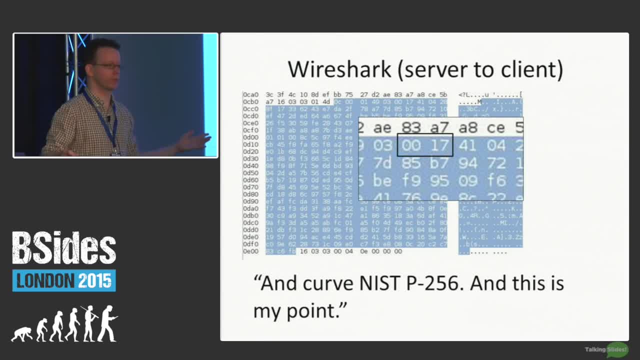 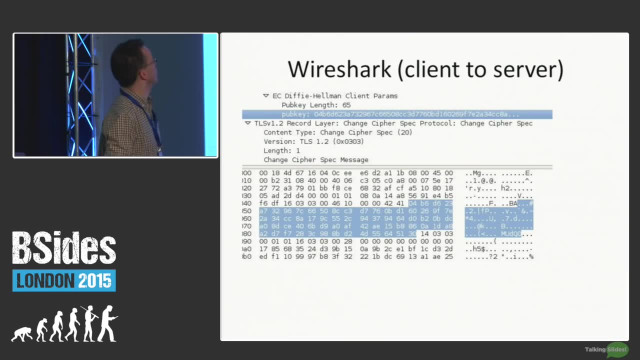 these are the bits of the. this is a number. It's actually the point on the curve that they're going to use. No, sorry, this is not. This is the B times B that's shared in the public point, And likewise, this is A times B. for what? 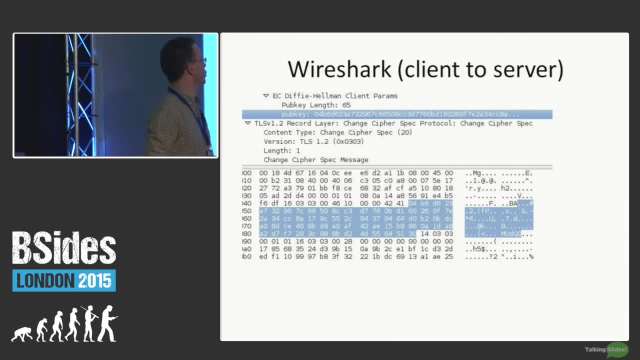 the client tells the server. I guess this is a bit confusing, to which I apologize for, But my main point I'm making here is: you can actually see this happen in Wireshark, And Wireshark more or less tells you what's happening. 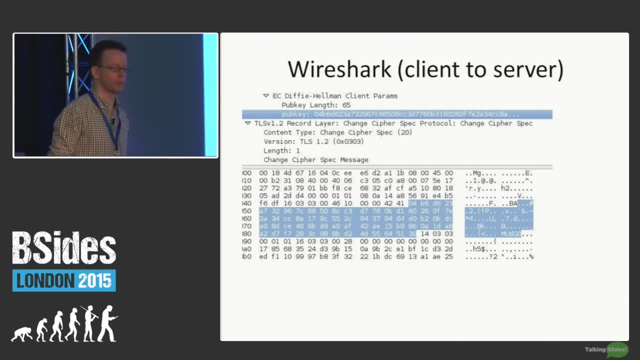 You can actually follow it. You don't have to understand the crypto, the math behind it, or you don't have to know all the standards, But Wireshark tells you all this. Here's my point. And now they have agreed on a shared number. 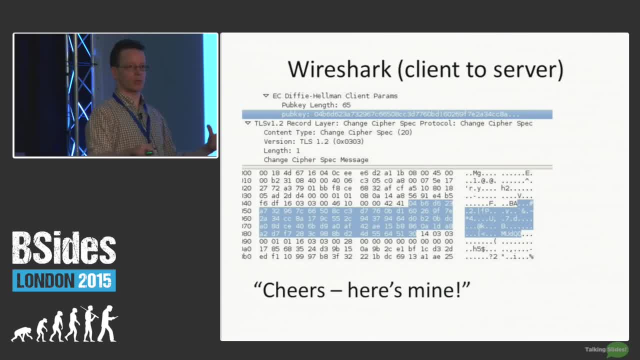 And you can't see this in Wireshark, because that's the whole point. I mean, Wireshark can see what Wireshark does- a man in the middle. but the whole point of ECTH is that you can agree on it. 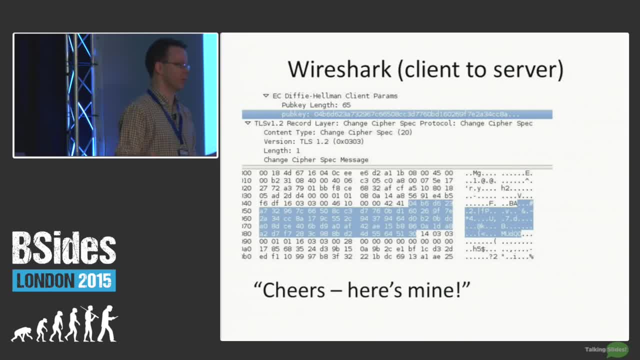 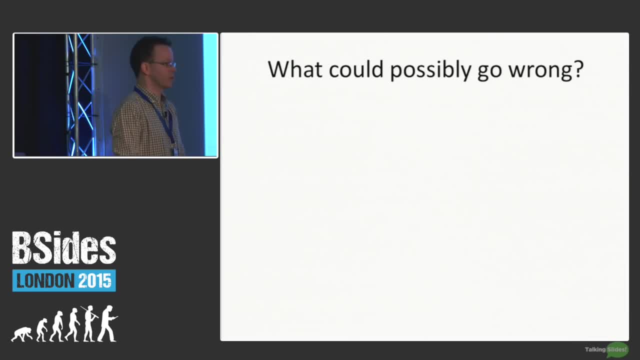 It's a secret number, secret key, while someone is listening in the middle. So what could go wrong? And there are a number of things that can go wrong- by choosing a wrong curve. As I said, there's a choice to be made for the curve. 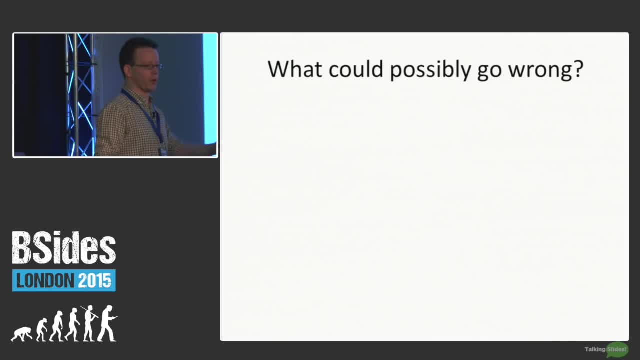 And there are good curves and bad curves, and good points and bad points. This is not a realistic example. This is something you can easily avoid, But just to give you an idea, I'm going to show you what could go wrong in theory. 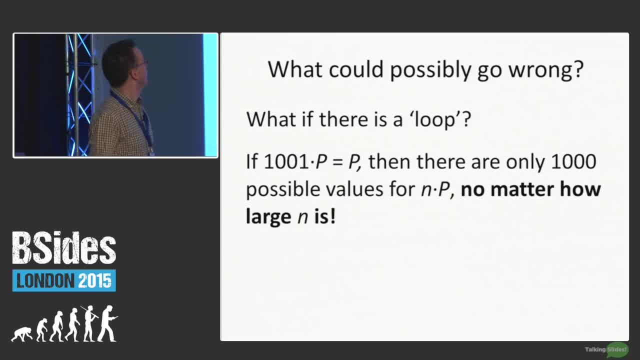 What if there's a loop? What if it happens that if you take this point P and you add it to itself, et cetera, and 1,001 times P is again the point P? I mean, it could happen. 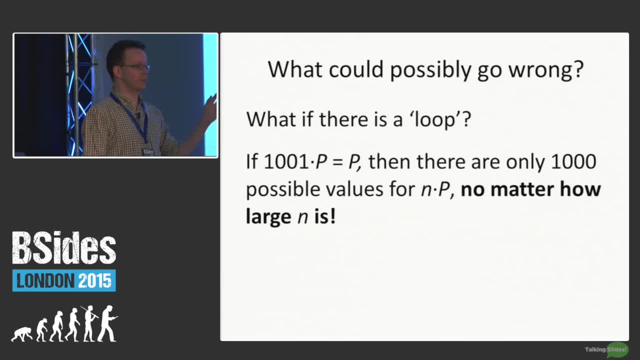 This means that 1,002 times P is 2 times P And 1,003 times P is 3 times P And a million and 1,001 times P is P. again, There's only 1,000 different values of P. 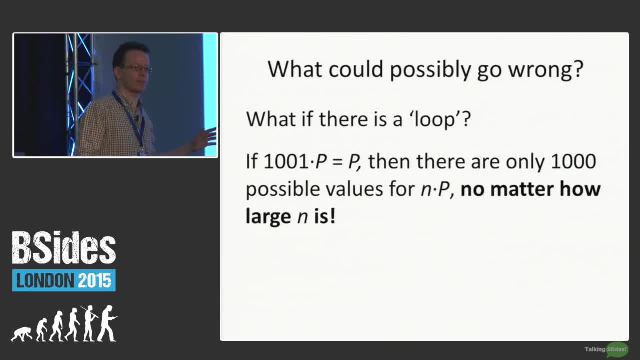 The algorithm still works, But someone trying to crack it has only have to try 1,000 different values for the points that they have to solve, which is trivial for a computer. And again, these kind of loops, they're easy to avoid. 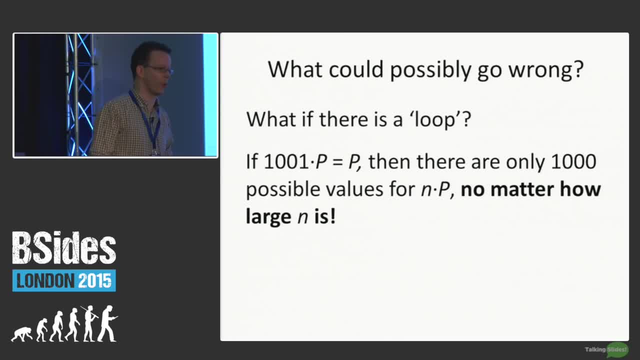 They don't happen. But this is the kind of thing that could, at least in theory, go wrong, And that's why you have to be careful. So loops can be avoided, But there's a large number of known weaknesses: curves you. 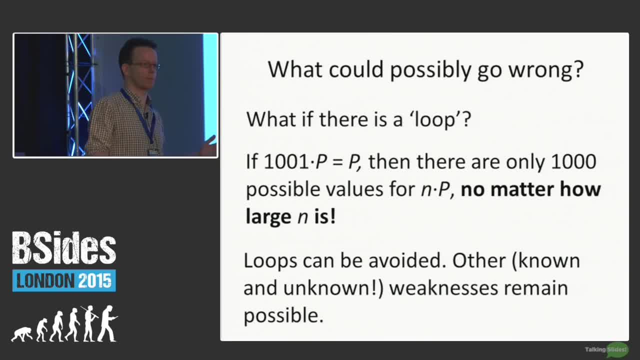 should avoid, And possibly there are unknown weaknesses, things that no one knows, curves that no one knows are weak, because no one knows the weakness, or curves that some secret agency knows are weak but the rest of us don't. So I showed in this Wireshark session. 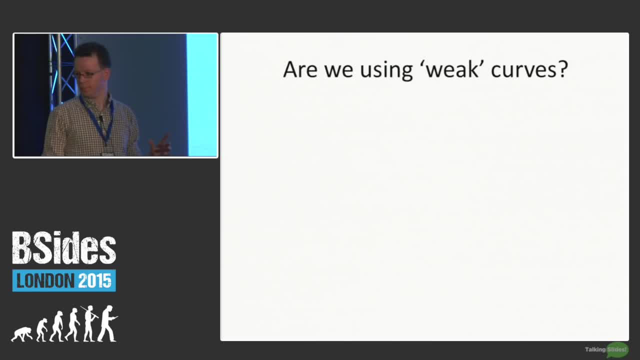 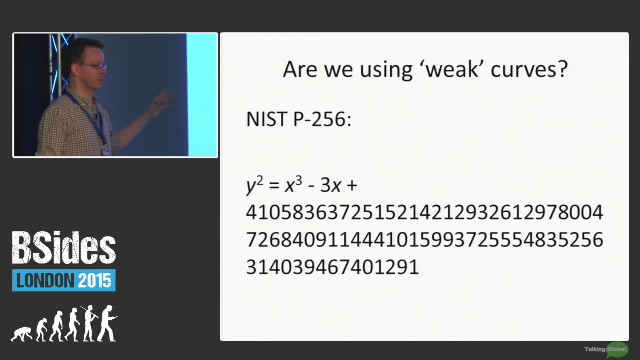 that we were using a curve called NIST P256.. It's defined as follows by this equation with a very large number. This is the kind of large numbers you see in crypto. That's nothing strange. So it doesn't refer to the fact that this. 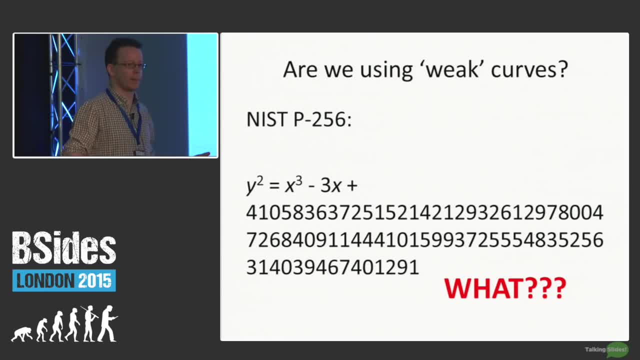 is a large number or a number that looks random. That's the whole point. But there is no good explanation of why NIST chose this number, this curve, which is a bit worrying. I don't think there's a backdoor or there's a secret algorithm. 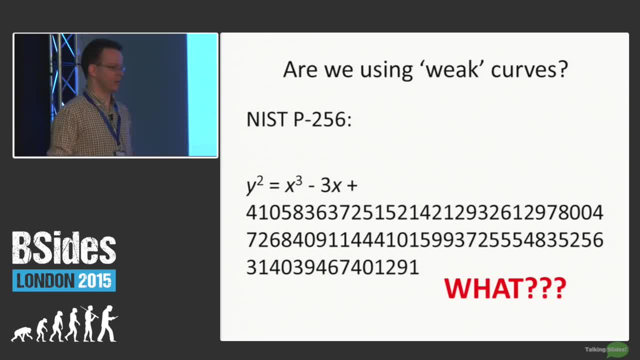 a secret weakness that NIST or their buddies at the National Security Agency know about, But it's a secret. It's possible And I think we should avoid this kind of curves, And it's kind of worrying that this happens between most elliptic curves. 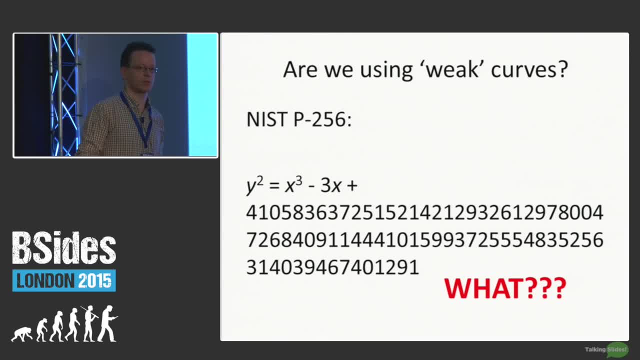 Crypto, when it's used to secure HTTPS, uses this kind of curves And it's kind of worrying that no one warns us about it. But people aren't- apart from some people on the IETF mailing list- people aren't really saying hold on. 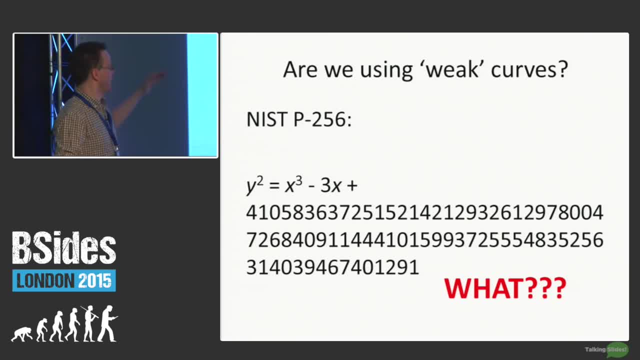 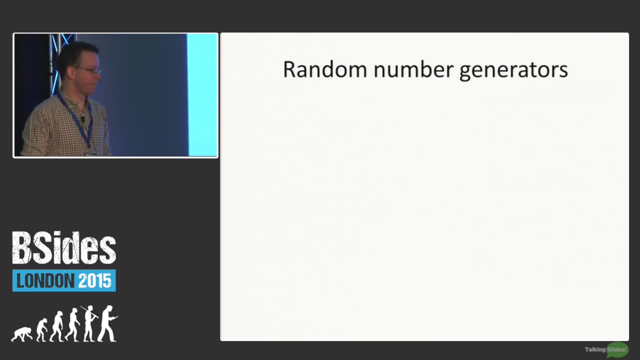 we should choose curves where we can explain all the. so we should choose curves where we can explain all the numbers. OK, There's another application of elliptic curve crypto that I think is interesting, And that's random number generators. I've mentioned the word random a few times. 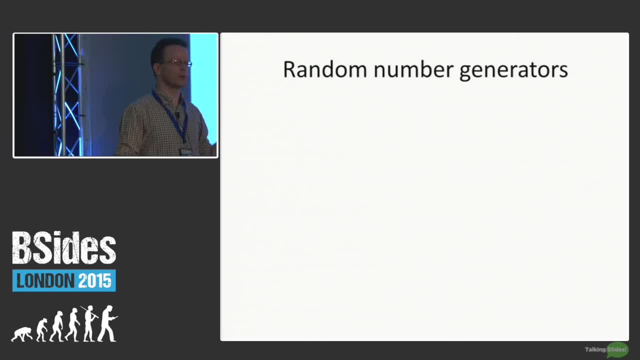 Alice and Bob needed to choose random numbers. People need to choose, or computers need to choose random numbers all the time And they need to be unpredictable and truly random. And that's hard because by nature, computers are good at doing predictable things. 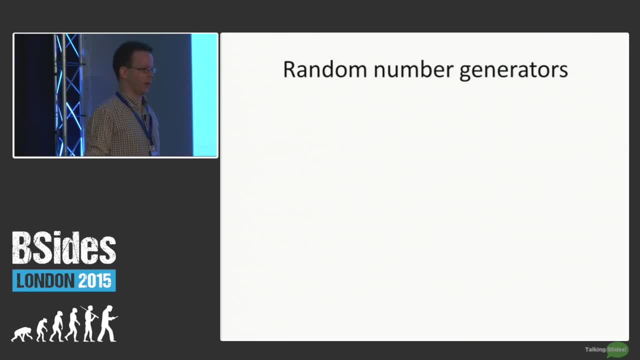 Thankfully, computers have a bit of randomness, Things like how long it takes to write things to a hard disk, how long the movements of the mouse. But that's never enough. Computers need much more randomness than that, So they use something called the random number generator. 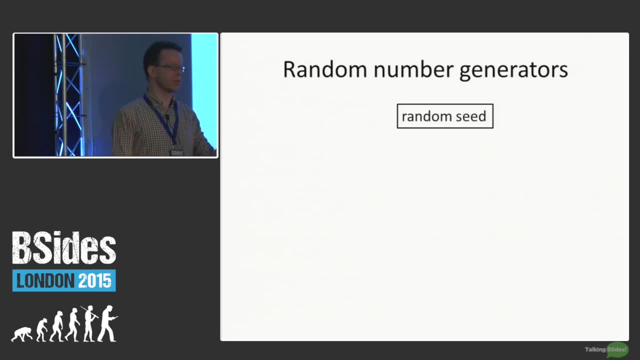 which is something that takes us to input a truly random seed, So something generated by moving a mouse, movement, hard disk read times, et cetera. Then it inputs it into some algorithm And some shaking up happens And it gives an output, a number: 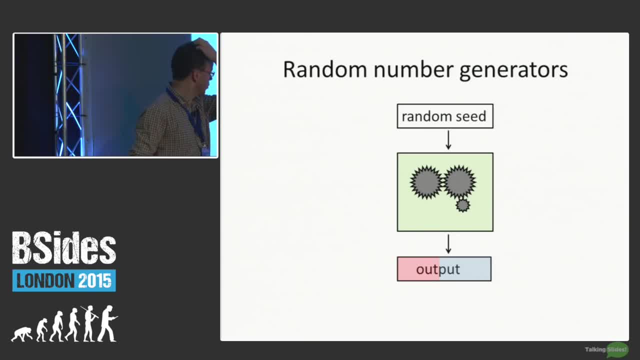 And sometimes- and this is why it's blue and red- sometimes part of the output is thrown away, And in this case, the blue output is the output of the random number generator, Whereas what was the internal state is shaken up again, And it's another output and another output. 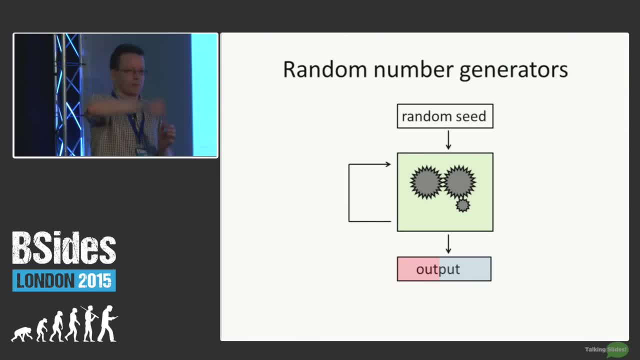 And I really imagine this, where you input a number and then there's some kind of churning and you churn out random numbers All the time, And this is what happens all the time in random number generators. This is how they work at the very basic level. 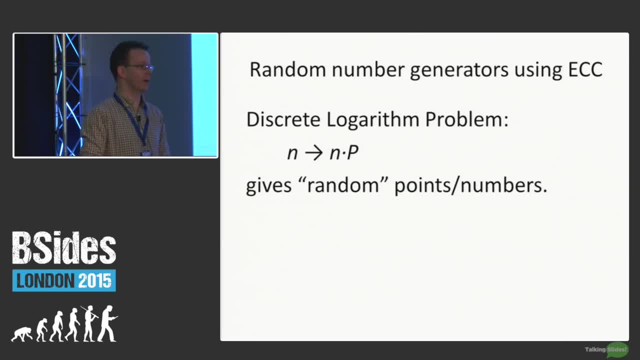 I mentioned the discrete local rhythm problem, which means that if you have a point n times p that you can't find the number n. So that's kind of useful for random numbers, Because you take the number n, which is, say, your random seed. 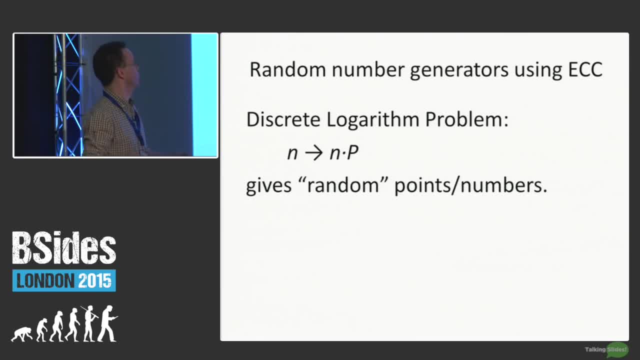 And you take n times p, which is a new point slash number. I said we could identify points and numbers, which looks really random, So you can make an algorithm where you start with a seed n0.. You take n0 times p. 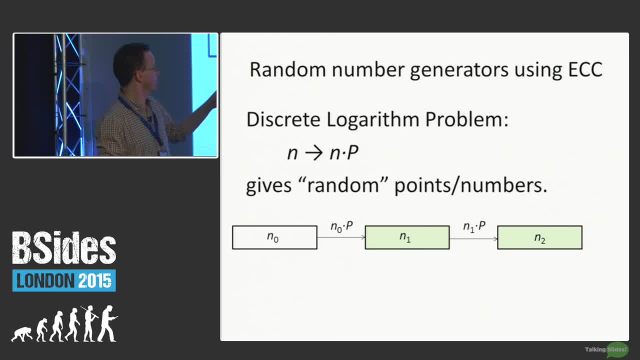 This is a number n1.. You take n1 times p, You get the number n2,, et cetera, And the output of the random number generator is just a series of n1,, n2,, et cetera. So you start with a random seed, n0. 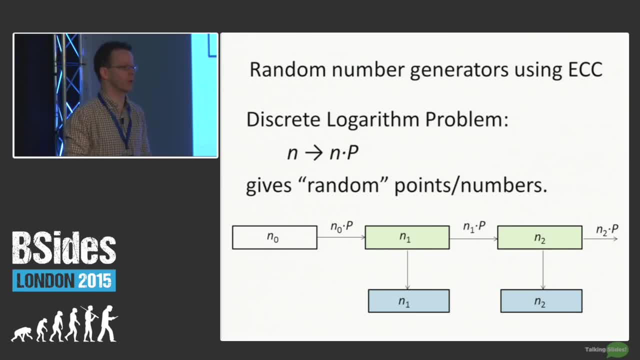 Using a point p on an elliptic curve and you get a nice random number generator. Well, there's one problem here. It is reasonable to assume that an adversary can read the output, Say they can read n1. That's not a bug. 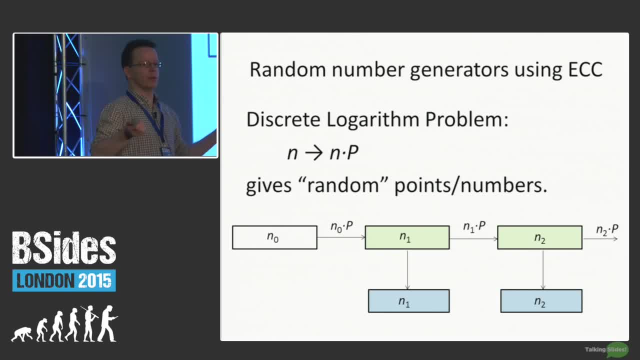 That's a feature of many random number generators. Random numbers are often shared. The problem is, if someone can read n1, they shouldn't be able to predict n2,, n3, et cetera. However, of course, if they can read n1,. 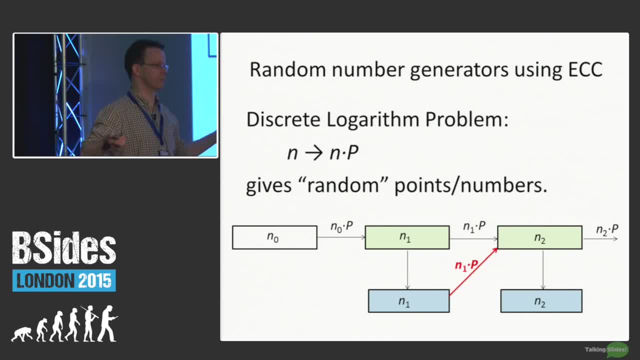 assuming this is a public algorithm, which algorithms should be in crypto, because we want things to be open. they can easily find the number n2,, n3, et cetera. So this is not a good random number generator, But you can modify this a bit. 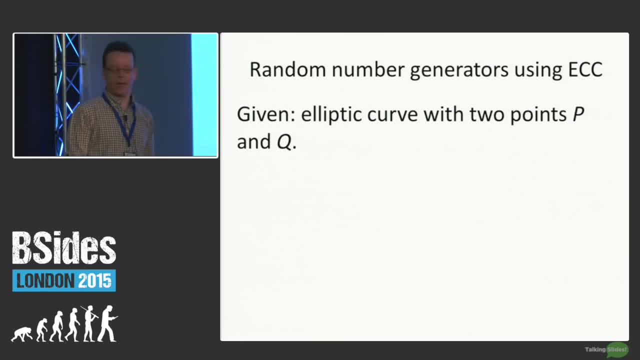 And we take an elliptic curve with two points on it: p and q, Two different points Again. Then we take a random seed. This is a real algorithm, so it's defined as a 32-byte seed- some random number. 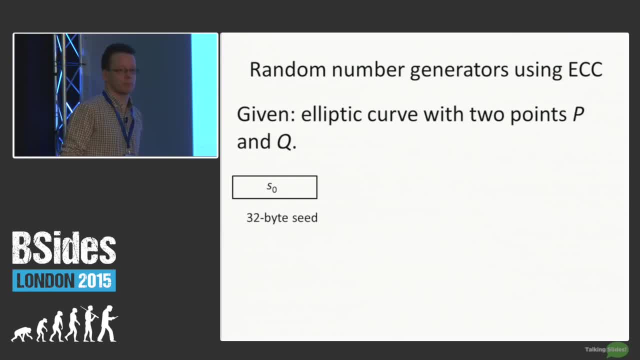 a truly random number called s0 in this standard, for some reason. And again, you take s0 times p, which is another number, slash point s1.. And what you then do is this number slash point s1, you multiply the point q by this. 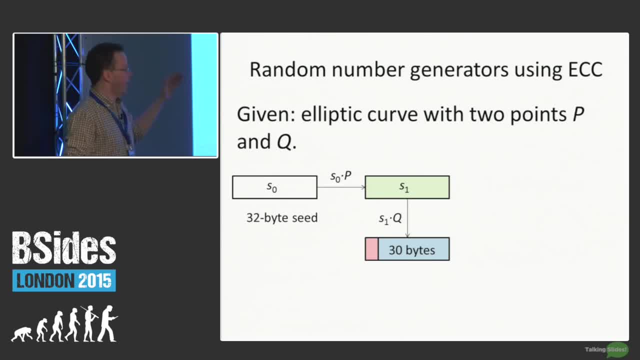 You get another number point, 32 bytes. You take the last 30 bytes, you ignore the first two bytes and this is an output of the random number generator. And again, with this s1, you multiply p with s1, get s2.. 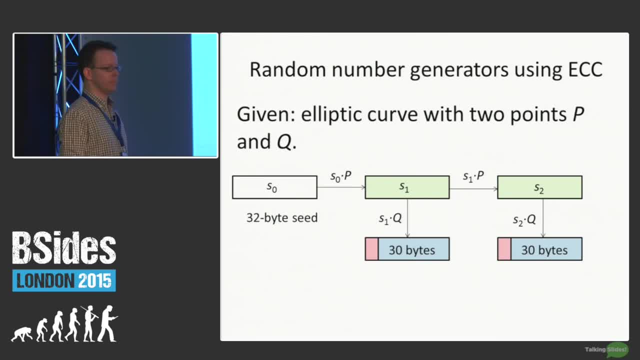 You get s2 times q, you get another random output, et cetera, Because knowing S1 times Q doesn't give you S1, that is the discrete logarithm problem. this is a good algorithm. This is a good random number generator. 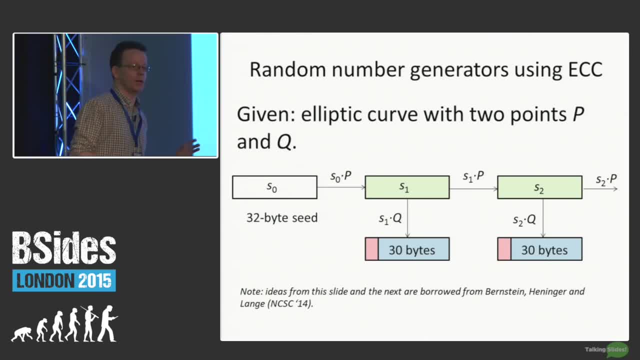 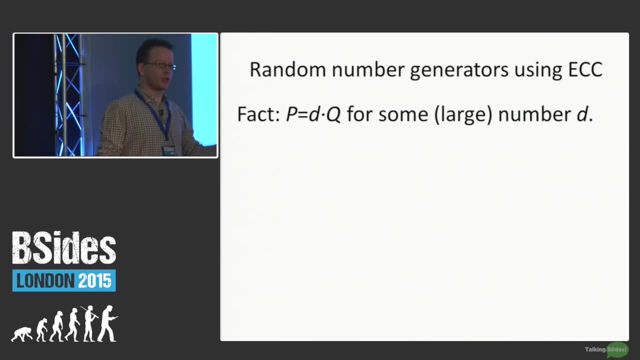 And I should point out that this and the next slide, the idea of this or the way to explain this, is borrowed from Dan Bernstein, Nadia Henninger and Tanya Lange at a NCSC press conference last year. Now we have these two points, P and Q, on the same curve. 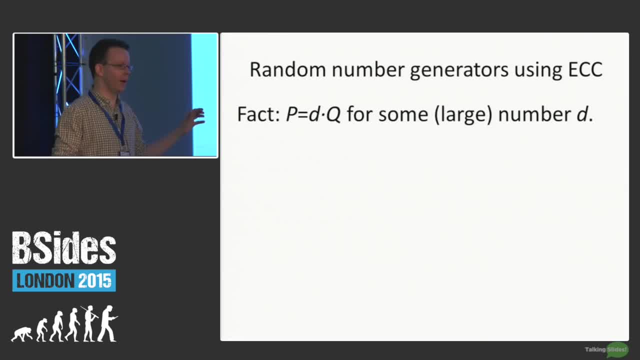 And for a fact, this is a known fact- about this curve, about many curves in general, there is a large number D, so that P equals D times Q. But you can't compute it because that's the discrete logarithm problem. 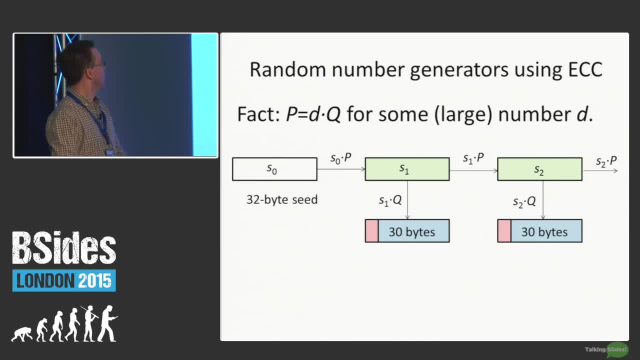 Now let's see. Now let's see. Let's show the algorithm again. This is the same as the previous slide, And also note that there are only 2 to the power 16 possibilities. So if someone sees the blue bit, the 30 bytes as output. 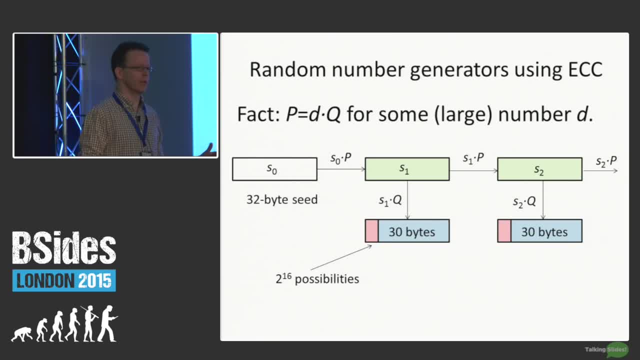 and again, that's a feature of random number generators. they sometimes see the output. then there are only 65,000 possibilities to get the whole output of S1 times Q And that's actually very easy to compute. because this needs to be computed. 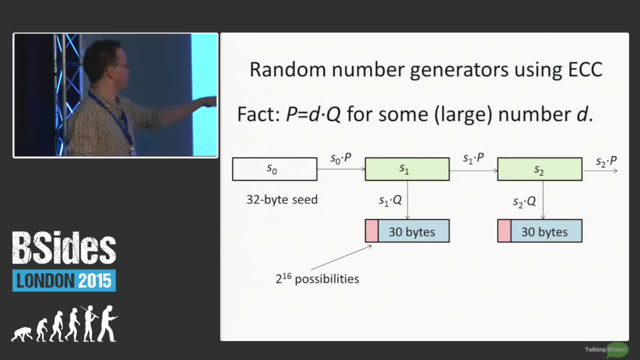 It needs to be a point on the curve And it's trivial to given the blue bit, it's trivial to find the red bit. And let's call this number R1.. This number which, again, can be easily computed, 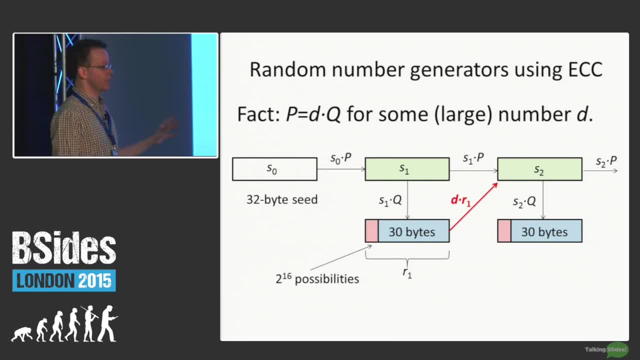 Now, imagine someone knows this number D. Imagine someone knows the secret number D. Someone somehow had access to it And again pointing out: you can't compute it. It's impossible to compute Now. now my claim is: if you take R1, which is publicly known, 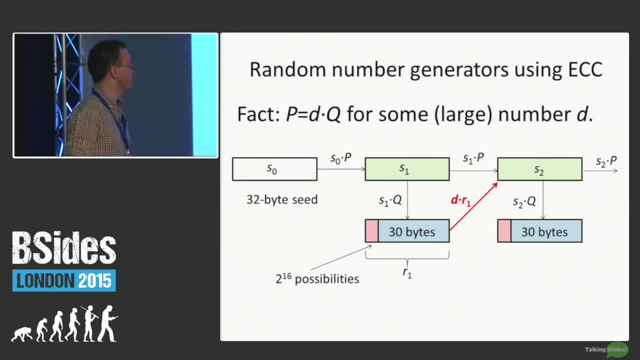 and this D, which is secret except for to this person or entity, D times R1 is the same as S2.. You can believe me that it's true, but I can even show it to you: S1 times P, which is S2,. 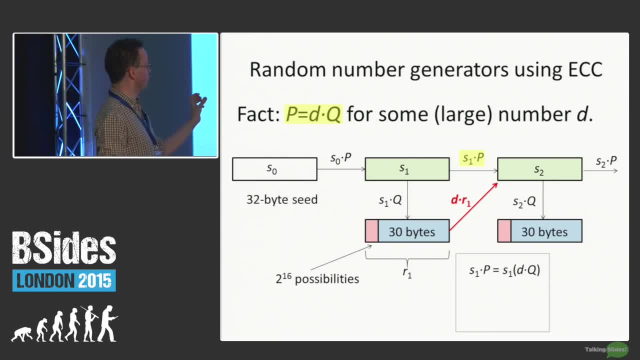 is the same, which is, by definition, S2, is the same as S1 times D times Q, combining the two yellow bits, because P equals D, D times Q. Because they work nice, you can change the order of D and S1,. 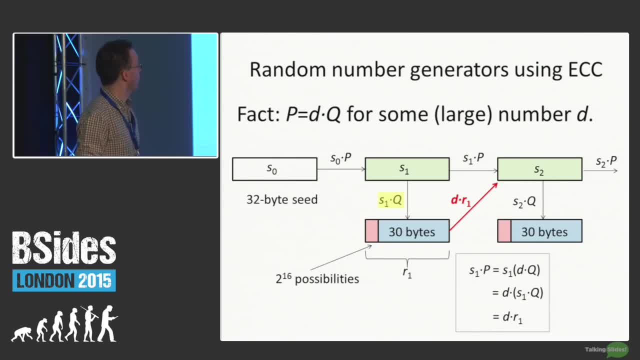 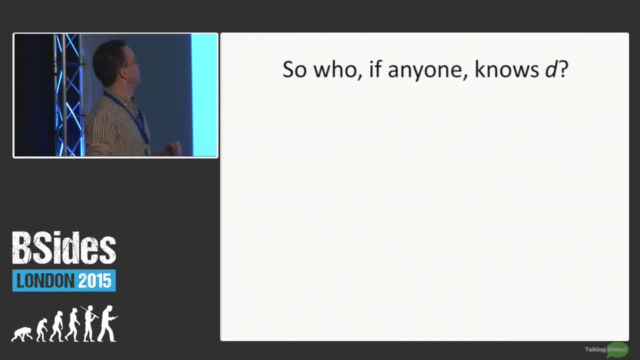 so D times S1 times Q is D times R1.. So I'll just show you that the red arrow indeed works. So if someone knows this number, secret number D, they can crack the algorithm. This is a. yeah, this is a big problem. 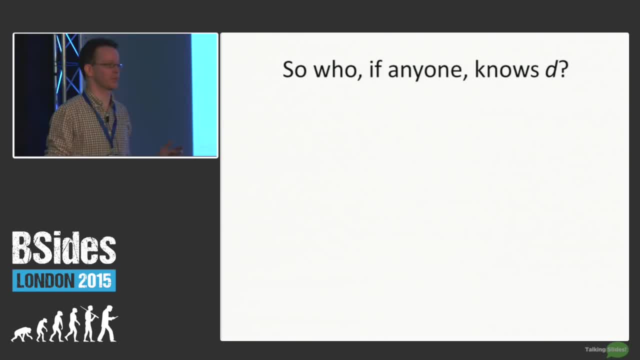 So the question, the million dollar question or the $10 million question- that's an in-joke- is: does anyone know this number D? Well, this is a. as I said, this is standard, It is defined. you can read it. it's defined by NIST. 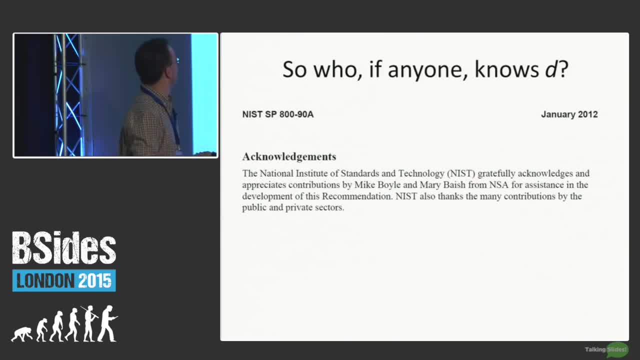 and helpfully. on the first page of the standard it has the following acknowledgment: NIST gratefully acknowledges that and appreciates contributions by Mike Boyle and Mary Bates from NSA. Oops, Oops. As many of you will have realized by now, 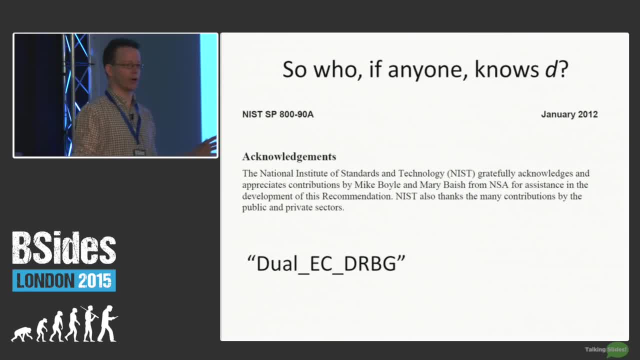 this is the infamous backdoor in dual EC DRBG- the random number generator. And this is just not just a theoretical problem. This random number generator was through some social engineering and $10 million made the standard in RSA crypto libraries: RSA as in the company, not RSA as in the algorithm. 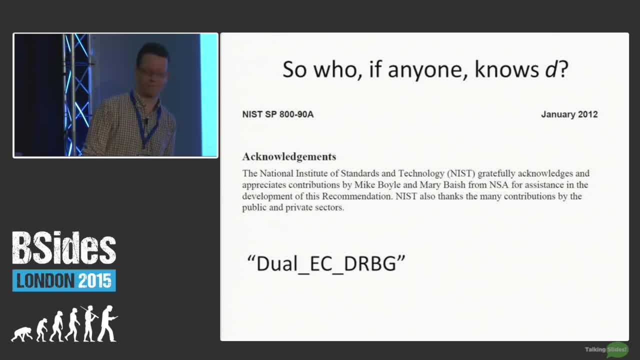 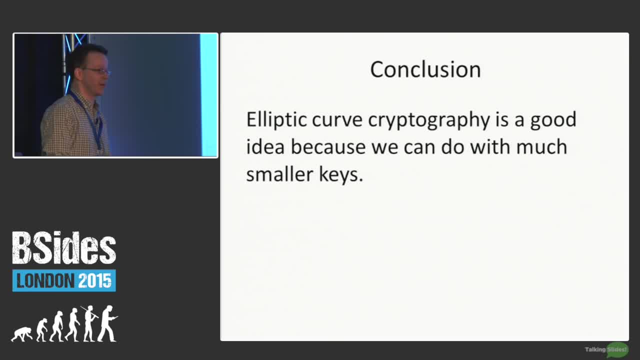 Right Conclusion. I haven't really explained this, but elliptic curve cryptography is is important because we can do it much. smaller keys, And that's that's the biggest, the main advantage. Keys of 256 bits give more or less the same security. 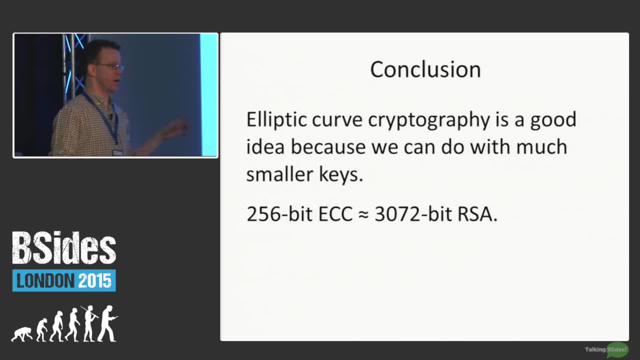 security using elliptic curve cryptography as 3072 bits RSA, and this also. they don't grow as fast, which means you can do shorter keys. algorithms are faster. this does make a difference as cryptos being widely deployed. there's one big weakness in elliptic curve cryptography: 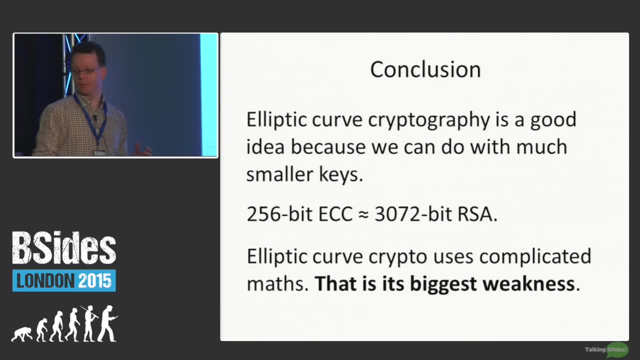 i think, and i don't think people realize it's enough. it uses complicated maths. it's great, it's fascinating, it's cool, but the fact that it uses complicated math doesn't make it stronger. ideally, you would have an algorithm that uses very simple math, that that anyone who could do a bit of. 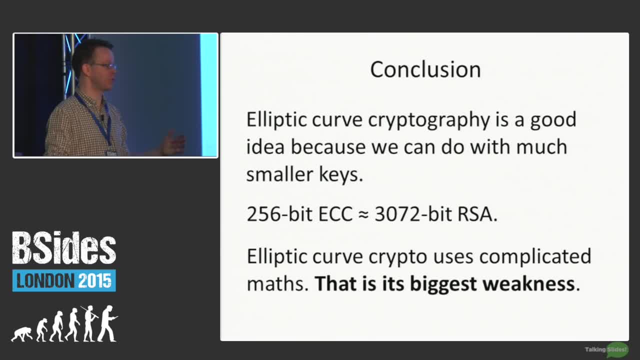 programming could understand, not something where we rely on a very small group of people who really understand this, hoping that they're on on our side, etc. and again, i'm not one of the people who understand this well enough to find algorithms, to find back doors, etc. i don't think the group of people who understand it is.